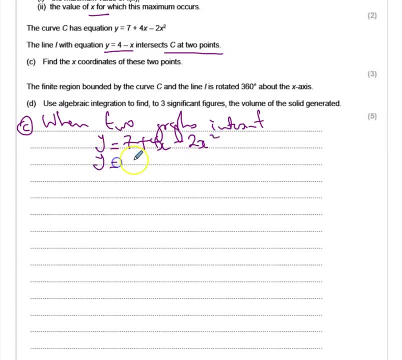 2x squared And we have y equals 4 minus x. Now, when they intersect, it means that there are two points, in this case because of the shape of the quadratic curve, where the linear graph, the 4 minus x, will intersect. To find that point, we want to. 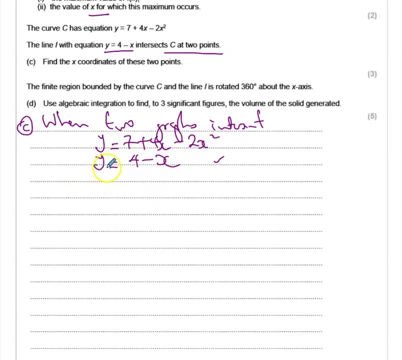 look at the position where they are both equal, because both equations have been written in the form y equals, y equals 7.. Now we can safely rewrite them as 4 minus x should be equal to 7. add 4x minus 2x squared, because after all they are equal. So now we can see a quadratic emerging here. 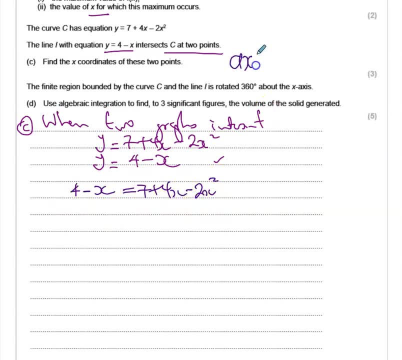 so we want to rearrange again so that we can achieve x squared plus Bx plus C, our almighty formula. Because I want to minimise the appearance of negative terms in my equation, I will be adding 2x squared to both sides and what else Subtract 4x from both sides, and then I will 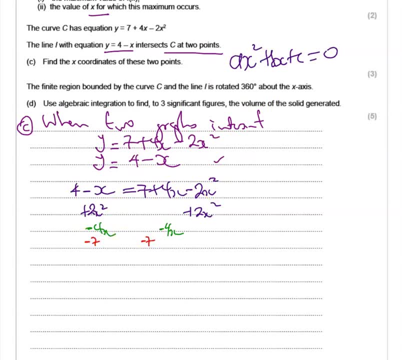 subtract the 7 from both sides. So once all that is done, my left hand side is going to look like this: So I have 2x squared, then I have my minus x. minus 4x will give me minus 5x, then I have 4,. 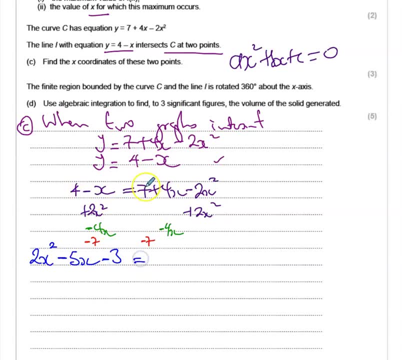 take away 7 gives me negative 3, and all of the right hand side would have been reduced to 0.. So now I need to factorise this equation. So I'm looking for two numbers, alpha, beta, So that the product will be 2 times negative 3, so I'm looking for the product being negative 6, but then their sum will be minus 5.. 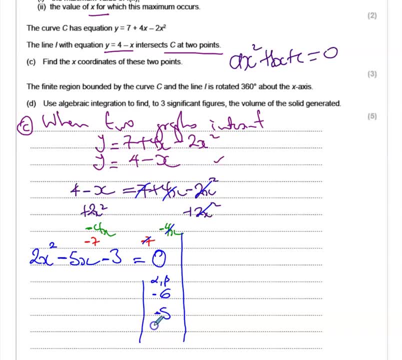 So, with a little think, you will be coming up with a 6 and a 1, and since we want to add them to get a bigger minus 5, so we would assign the negative to the 6.. So we have now 2x squared minus 6x. add 1, x minus 3, equal to 0.. 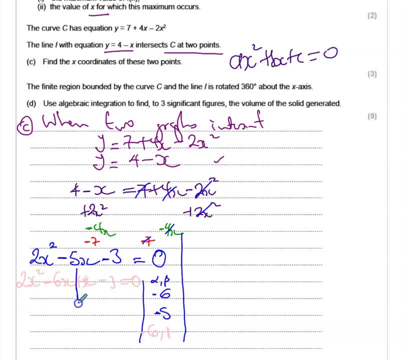 Let's try and factorise that. so if I put my curtain down here, I would have 2x as a common factor on the left hand side, with x minus 3 in the bracket. Now, whatever I get in the bracket here, 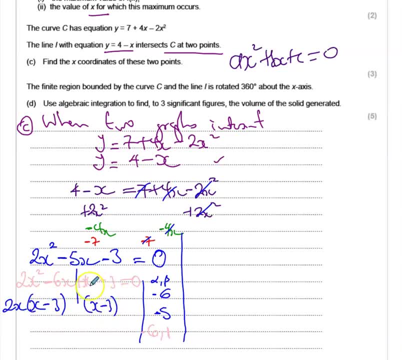 it will be the same thing I get here, so you can actually just repeat that and figure out what should go out to make the value a plus 1 when you multiply. and that should be it Now. x minus 3 here is a common factor, leaving us with 2x add 1 for our second bracket. 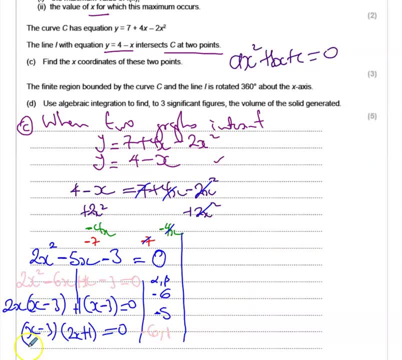 So again we do what we do best. We have 2 numbers multiplied. We are multiplying to give us a 0, so that means that either x minus 3 is 0, or 2x add 1 is 0. 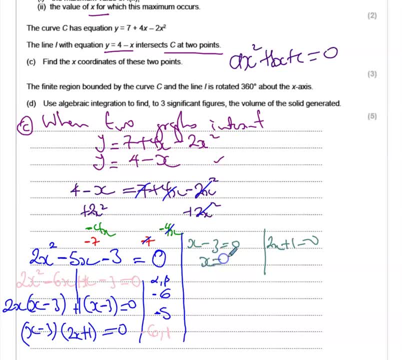 Now if x minus 3 is 0,, meaning x should be 3, and in this case 2x should be equal to negative 1, and therefore x will be minus 1 half. So now we have the x coordinate of the point where the two graphs intersect. 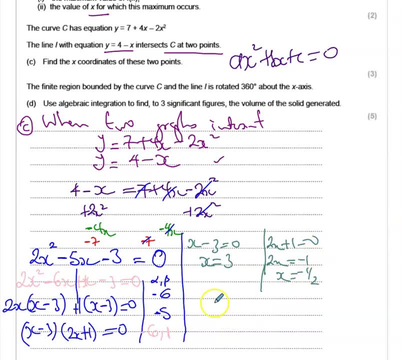 We now need to find the corresponding y value at that point. So we say y will be. I will be using the linear function because that's easier. You could also use a quadratic, it doesn't matter, you should arrive at the same answer. 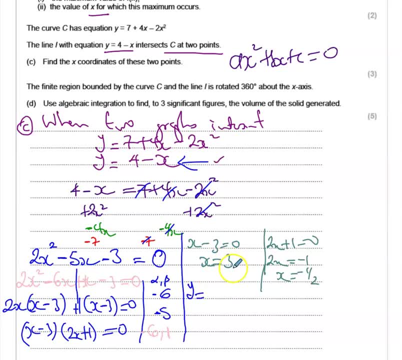 So in place of x I will be substituting 3, so I have 4 minus 3, and that gives me 1.. And what about the other side? I have x to be minus 1 half, so my y will be 4 minus minus 1 half.